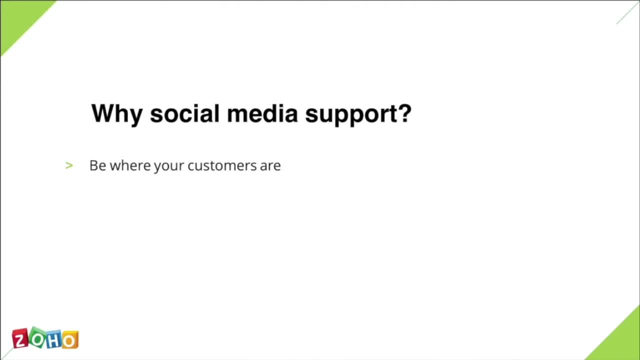 it make sense to offer support where your customers are. The usage of social media is increasing among all age groups, so make customer support as easy as pinging a friend for help. But social media support doesn't just benefit your customers. it can also make your support. 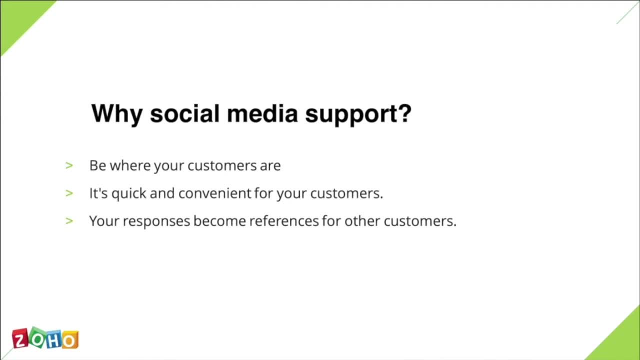 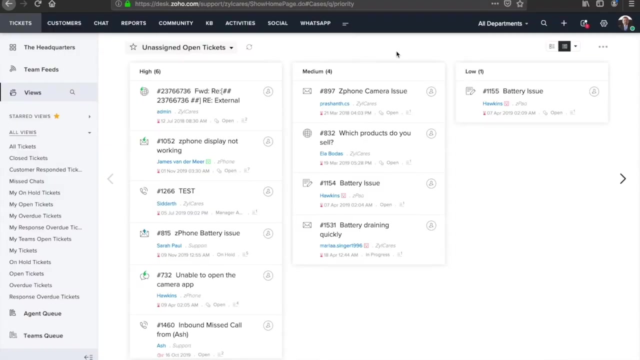 more efficient. Unlike traditional support channels, your responses can be references for other customers. Social media is mostly an asynchronous communication medium, so social media support isn't as cost-intensive as synchronous support channels such as live chat or phone support. To link your social media pages with Zoho Desk, go to Setup Here under the Channels. 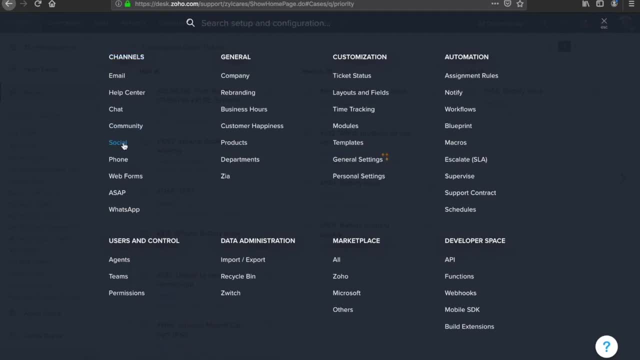 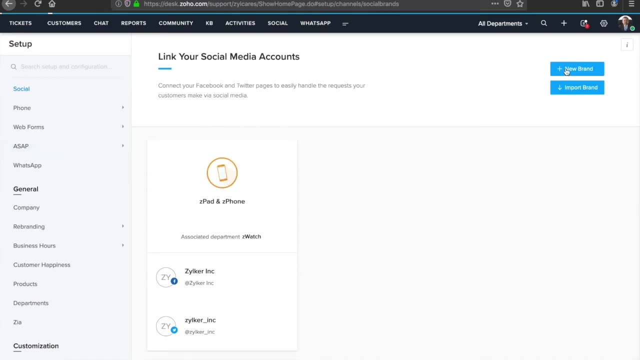 tab, select Social. Now, at the top right hand corner, select New Brand. Give the brand a name. Here you can associate this brand with all departments. Give the brand a description and click Save. Now that I've created a brand, I'm going to link my Twitter page with it. Provide your Twitter credentials and click Save. 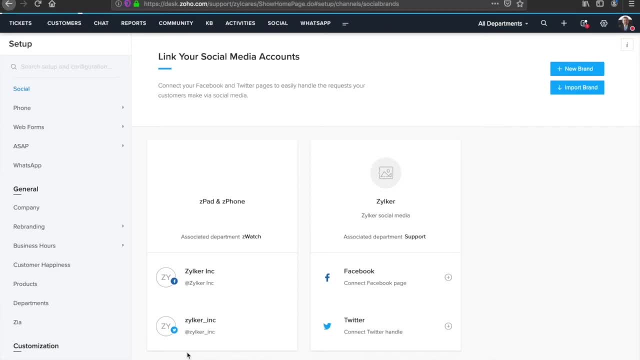 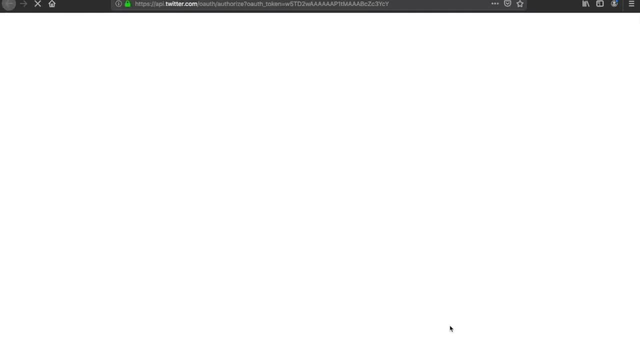 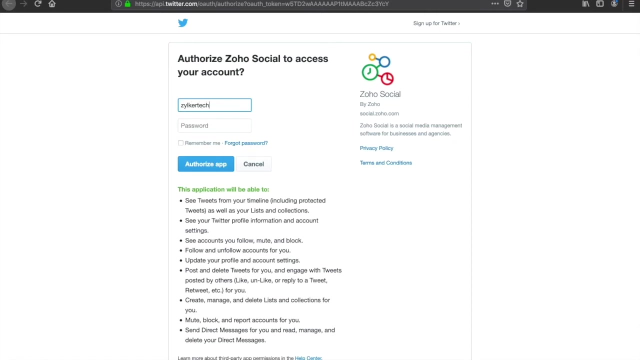 Now that I've created a brand, I'm going to link my Twitter page with it, Provide your Twitter credentials and click Save. Now that I've created a brand, I'm going to link my Twitter page with it, Provide your Twitter credentials and click Save. 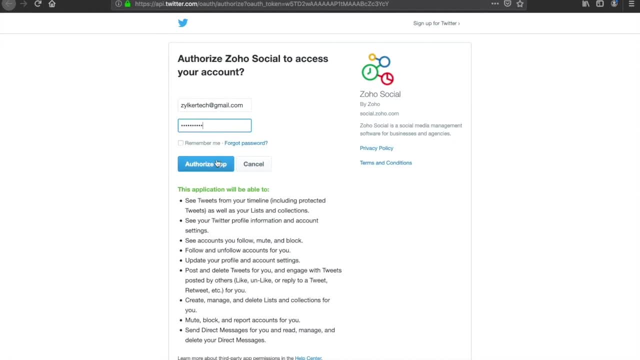 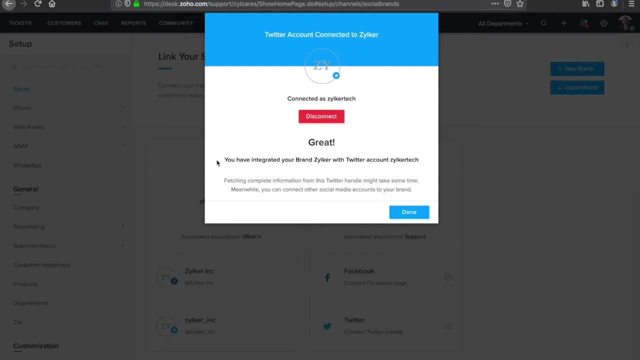 Now that I've created a brand, I'm going to link my Twitter page with it. Provide your Twitter tags and click Save And select Authorize App. Select, Authorize App. And now you've linked your Twitter page with your brand. 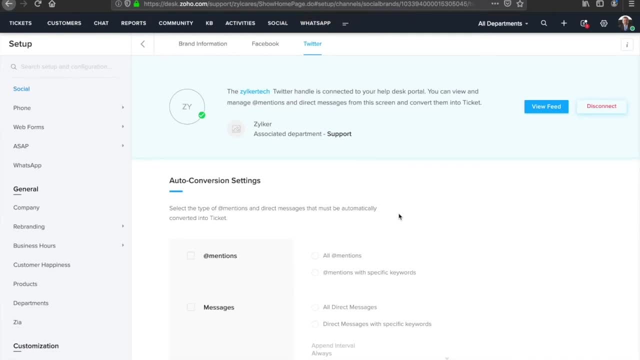 And now you've linked your Twitter page with your brand. Zoho Desk also lets you auto convert your apps, messages, mentions and posts from your social media. Here I'm gonna convert all mentions and all messages into tickets. It also provides you the option of a 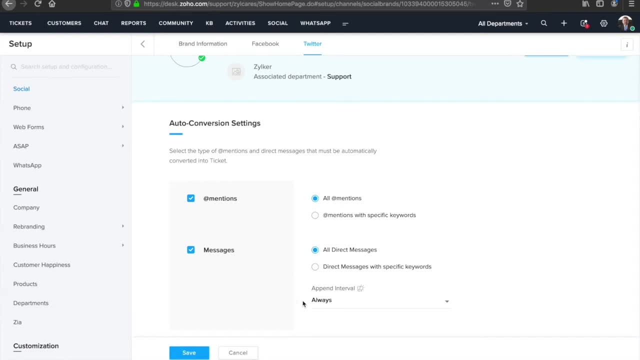 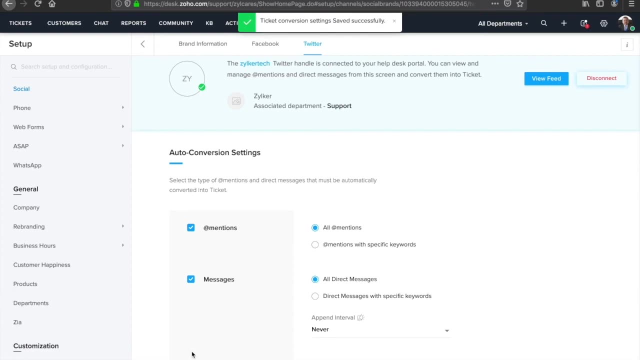 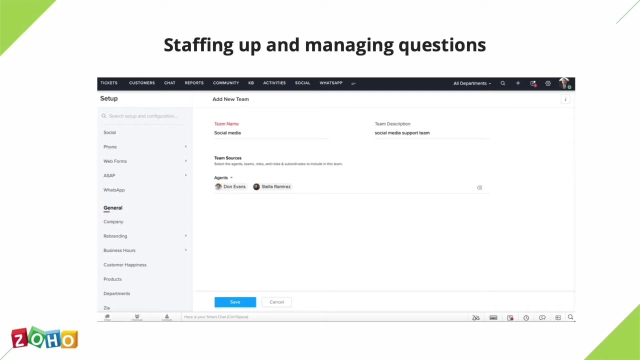 pending interval between tickets: Click Save. Social media support requires quick responses and accurate resolutions. Designate your best agents to handle social media requests and create a social media team so they can collaborate better. Creating a team will also let you assign tickets to these agents through a single direct. 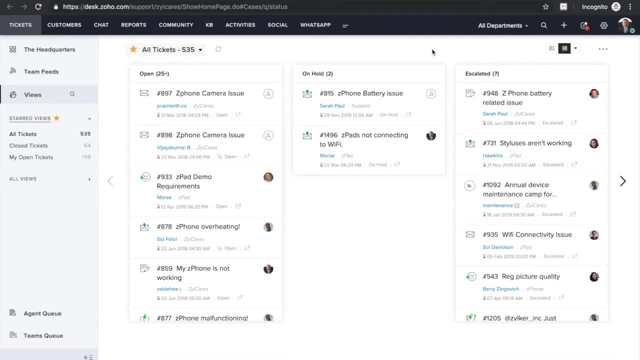 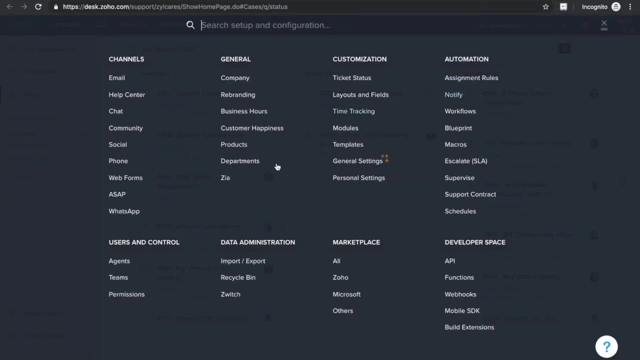 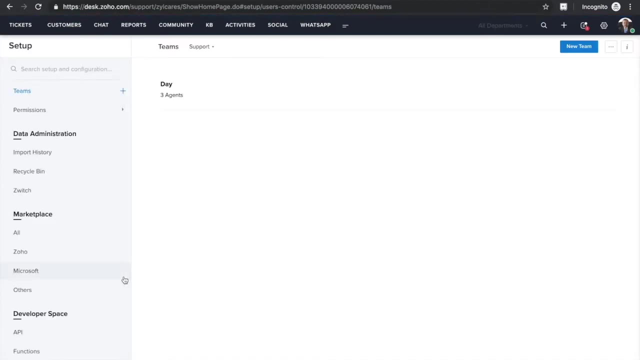 assignment rule. In order to create a team, go to Setup, Click Save Under the Users and control tab. select teams. First select the department you want to associate with the team. Now click on New team, Give this team a name and also provide a description. 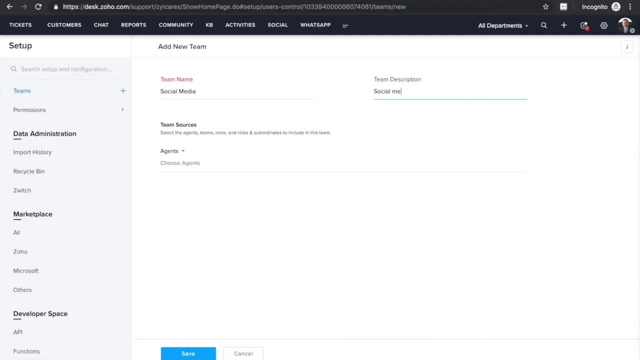 Now select the agents you want to add in the team. Click save. To create a new direct assignment rule. go to setup. Here under the automation tab, select assignment rules. On the top right hand corner, select new direct assignment. Give the rule a name. 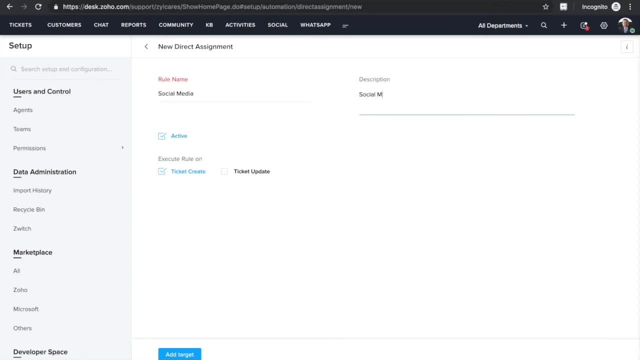 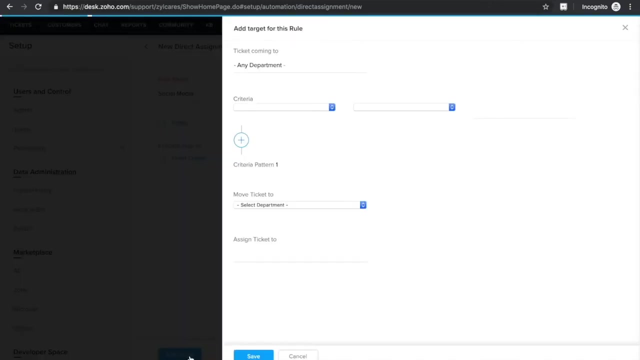 And also provide a description for the rule. Ensure the ticket create checkbox is selected. This ensures the assignment rule is triggered once the ticket is created. Now select add target. Ensure that any department is selected in the ticket coming to drop down. Now configure the criteria accordingly. 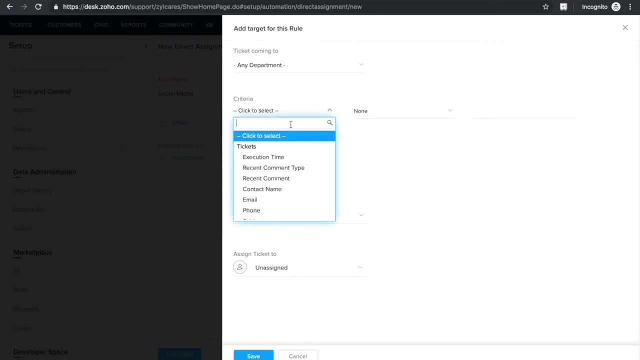 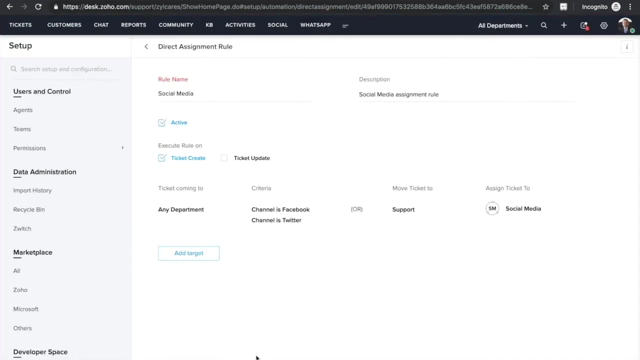 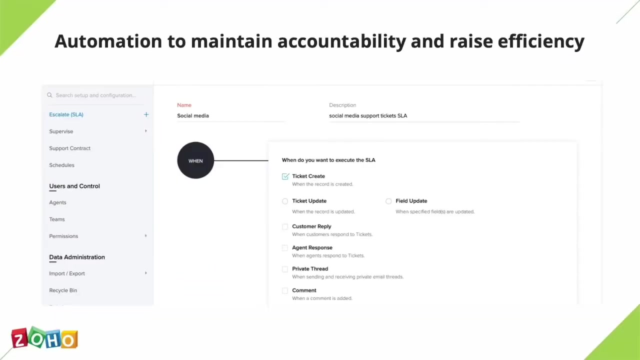 🙏🙏. Now select the department you want to move. the ticket to Click could not be added to the department. Now select the team you want to assign the ticket to Click save. It is important to ensure that social media tickets don't slip through the cracks and 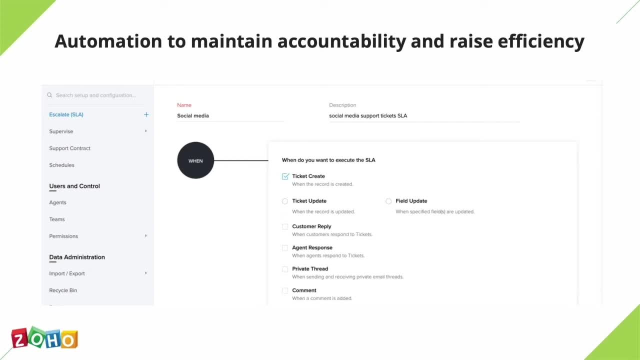 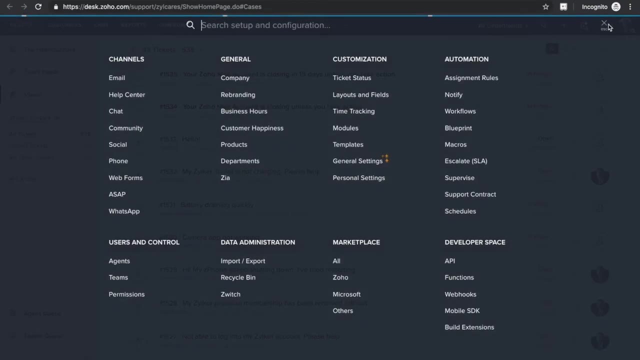 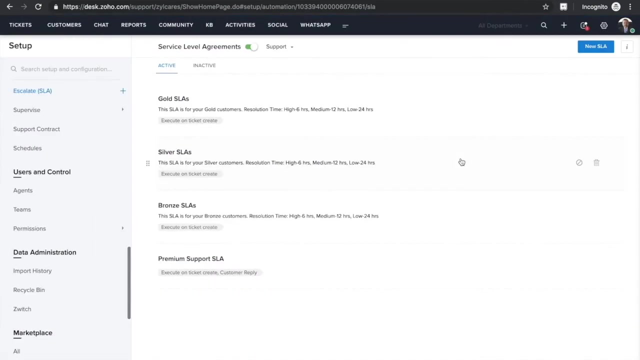 are responded to and resolved promptly. You can use service level agreements to ensure standards are met when it comes to handling social media requests To create a new SLA. go to setup Here under the automation tab select escalate. First, select which department you want to associate this SLA with. 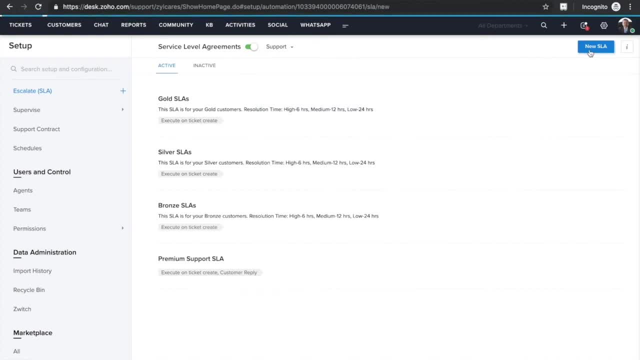 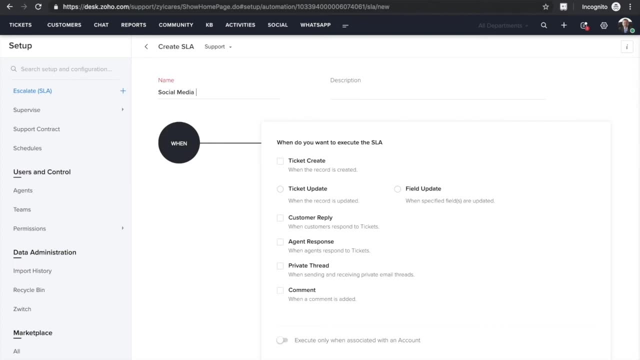 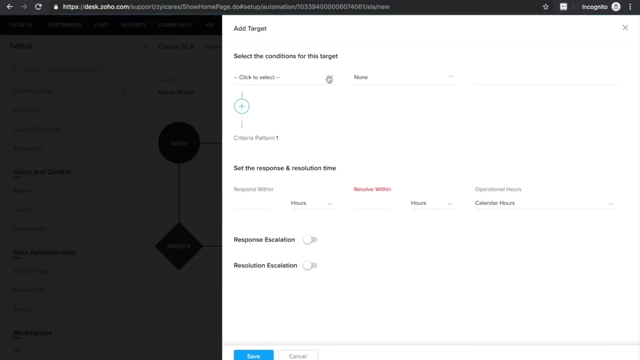 Then click new SLA. Give this SLA a name and also provide a description. Now ensure that the ticket create checkbox is selected. This ensures that the SLA is activated once a new ticket is created. Now select add target. Configure the conditions accordingly. 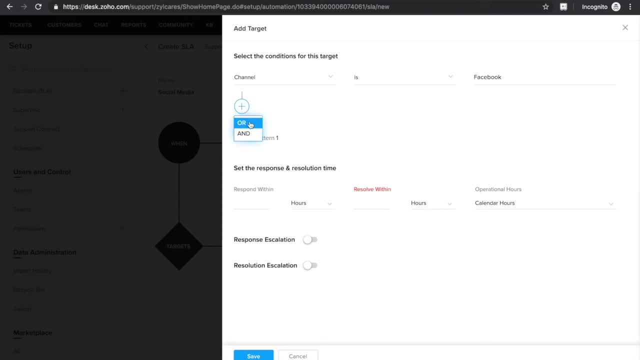 This gives you a new SLA and a new service line. Now set the response and resolution times. You have an option of triggering the SLA based on calendar hours or business hours. Lastly, you can also set the time, to select the date and time of obligation. 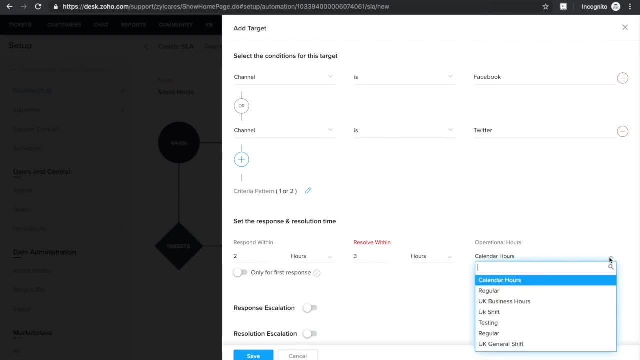 The next step is the trigger time. You can scale the trigger time for the SLA to match with the trade-off time as well as the time for which you want to trigger the SLA. To do this, you can select sll vad. 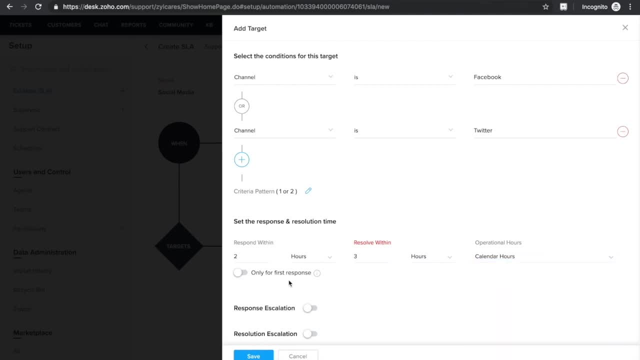 Click okay, You can also trigger the SLA just for the first response. Now slide this button to set the response escalation. First, select when exactly you want to trigger the SLA. Here you can either choose to escalate agents or teams. 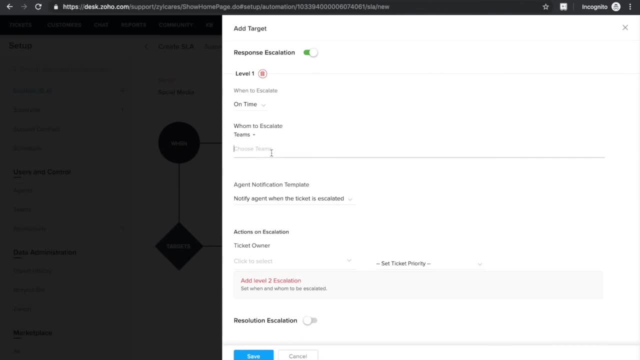 Here you can also decide when a notification is sent to an agent or a team regarding the escalation. Now select the new ticket owner after the escalation happens. In this case, it's going to be my support manager. Now slide this button to set the resolution. 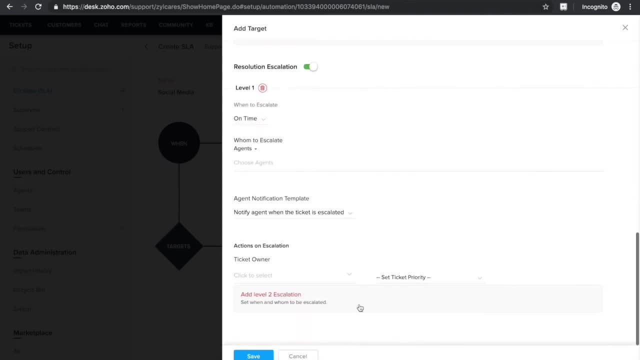 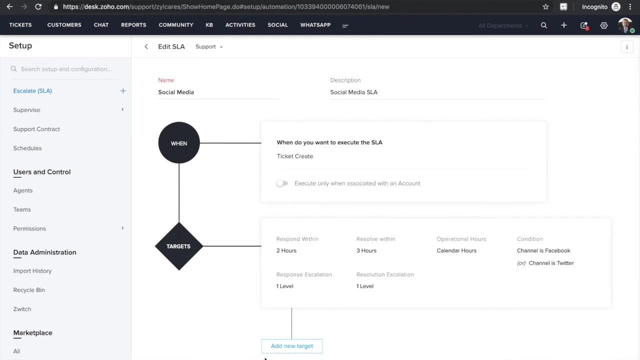 Here you can also set the resolution escalation. Here I'm going to escalate my support manager And the new ticket owner is going to be my support head. Now click Save. Monitoring metrics is key to understanding your support process and optimizing it. 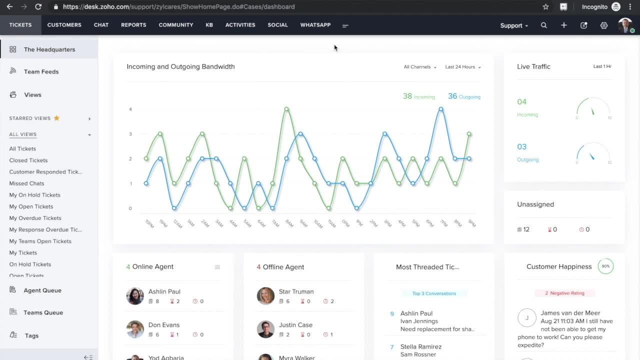 The HQ dashboard gives you a quick overview of ticket bandwidth and lets you plan and allocate resources accordingly. But if you want to view just your social media tickets, you can create a custom view. To create a custom view, select Views, Click on the plus button. 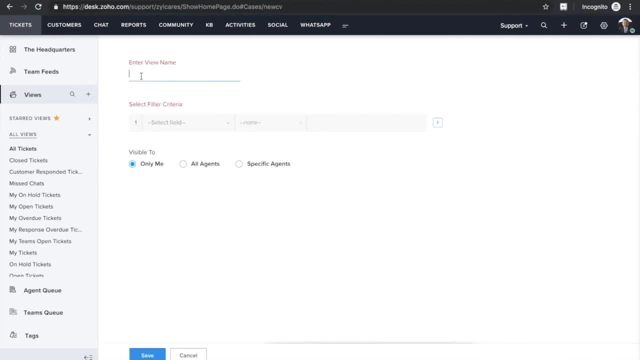 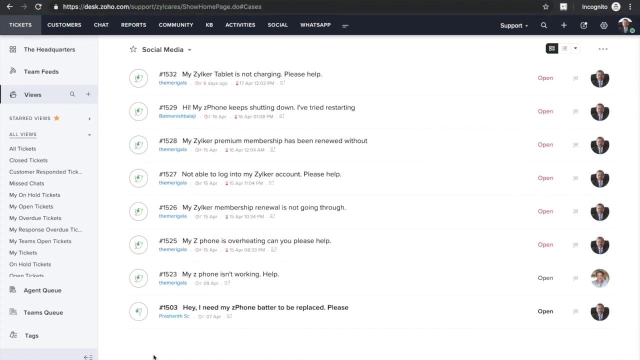 Now give this view a name and configure the criteria accordingly. Now select the visibility of the view and click save. There are many dashboards and reports that you can view, configure and even schedule in Zoho Desk, But the dashboard which is by far the most useful is the SLA dashboard.